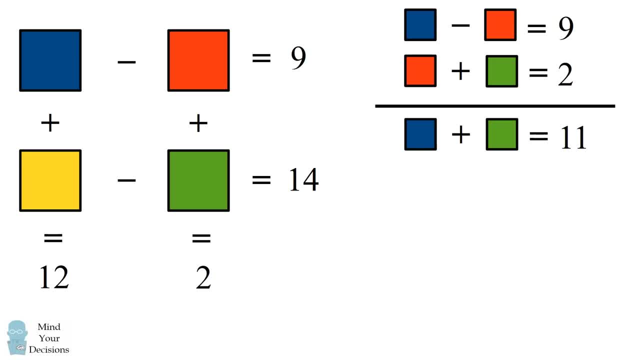 We can add up these two equations to conclude that blue plus green is equal to 11.. We can then look at the first vertical equation to say: blue plus yellow is equal to 12, and we can look at the second horizontal equation to get negative yellow. 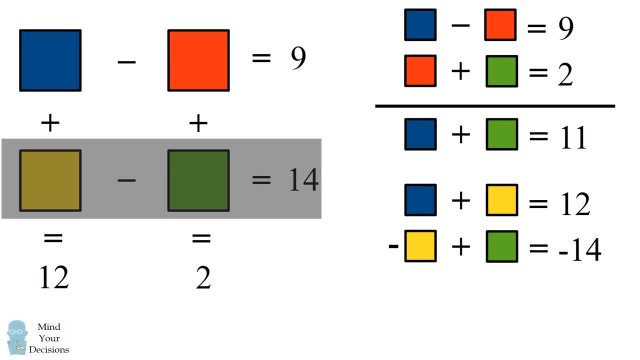 plus green is equal to 12. Plus green is equal to negative 14. I've multiplied the second equation by negative 1. This is so that we can cancel out the yellow variable, and then we get the result: blue plus green is equal to negative 2.. 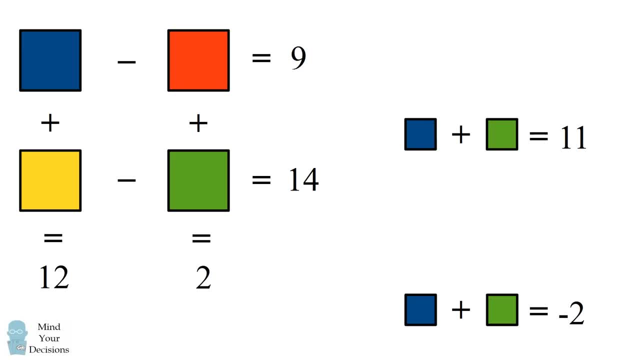 Now, if you focus on the two results we have, we have something that's contradictory. In one case we have: blue plus green is equal to 11. In another equation, we found blue plus green is equal to negative 2. It's not possible for these both to be true at the same time. therefore, we're 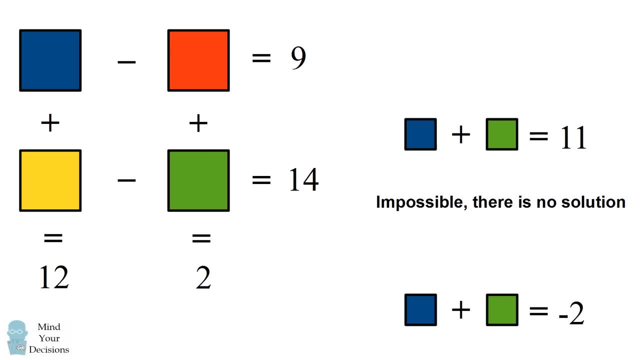 we've reached a contradiction and therefore this is impossible. There is no solution to this equation, to the system of equations. Now you might ask yourself: is it just because we had the numbers 9, 14, 12 and 2? is it possible that this system of equations could have another? 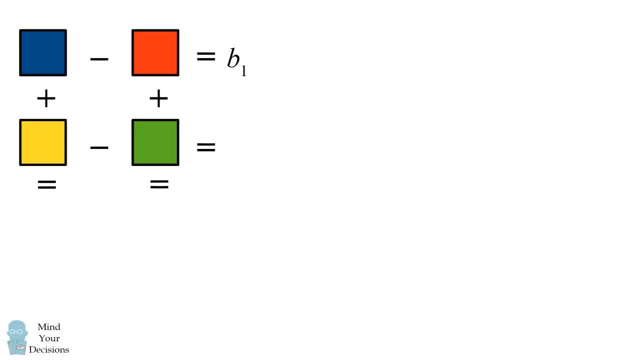 solution if we put different numbers, So if the first equation was equal to b1,, if the second horizontal equation was b2,, if the first vertical equation was b3, and if the second vertical equation was b4. Is it possible? Could we actually figure out a solution? 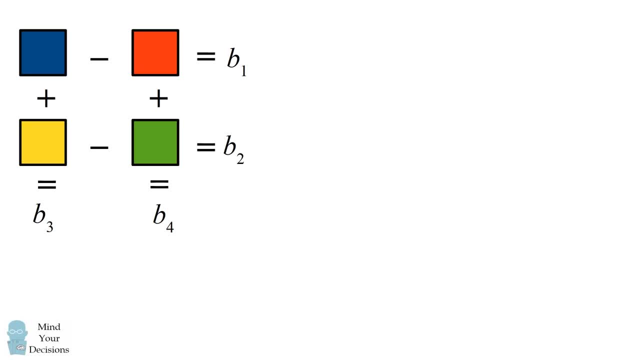 This is the type of problem that you would deal with in linear algebra. The result would be a vector of four variables: b1,, b2,, b3, and b4, and these are constants which are known. This is going to be the result of four equations, four variables, which is blue, red. 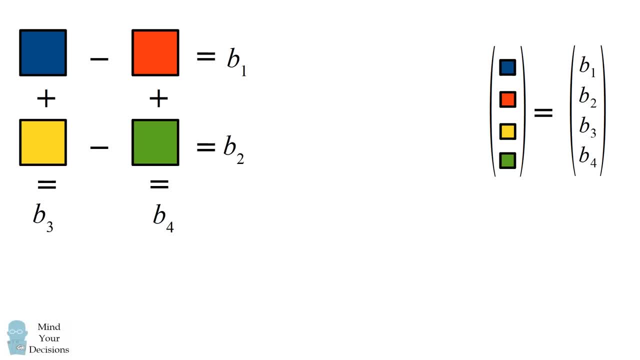 yellow and green. We can represent the system of equations by a linear operator which we can write as the following matrix: If we multiply the matrix by the vector of variables, we end up with the results. So the first line of the matrix says: blue minus red is equal to b1.. 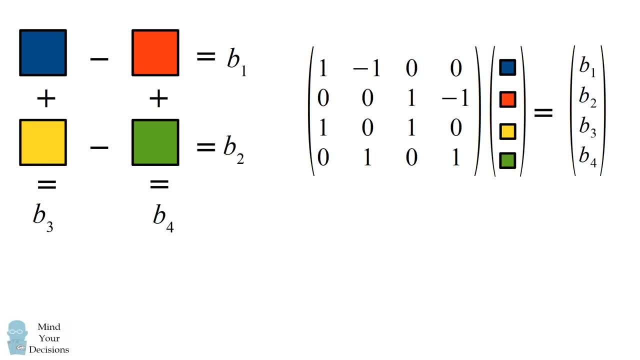 The second line of the matrix says: yellow minus green is equal to b2.. The third line says: blue plus yellow is equal to b3, and the fourth line says red plus green is equal to b4.. So we can write the following matrix: